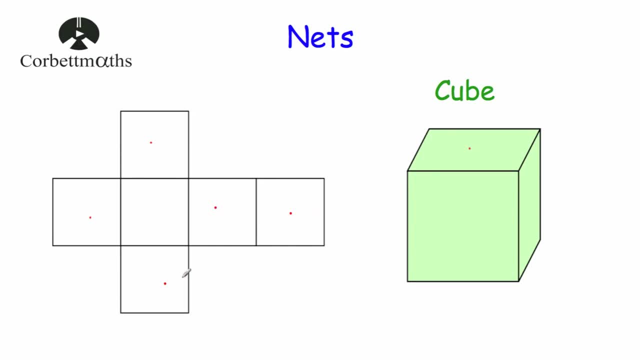 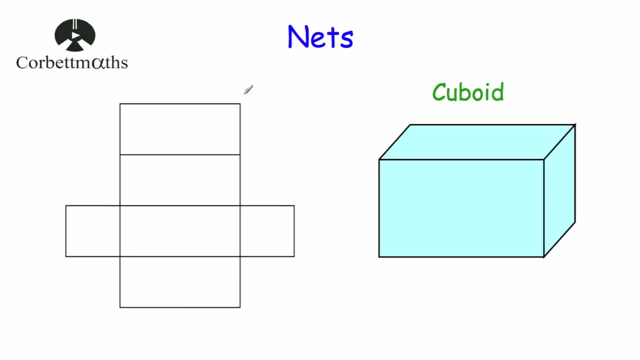 the lid of the cubes. Okay, so this is the net of a cube, and it's very useful to learn that and to know what that looks like. Now, there are different versions of the net of a cube, but this is quite a common one. Okay, let's have a look at another 3d shape. Okay, let's have a look at our next 3d shape. 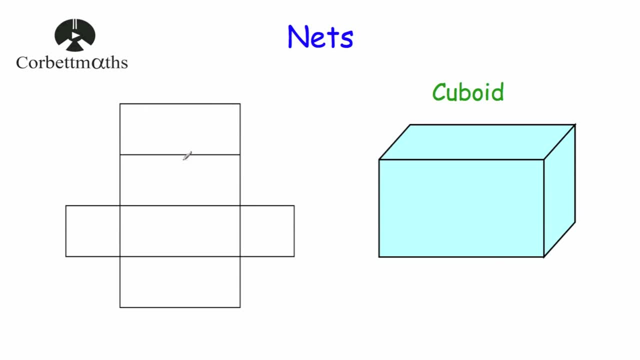 so we've got a cuboid, and the net of a cuboid would look something like this. Now, depending on the cuboid, it may consist of six rectangles, or it might have squares, such as this one that's got a square on the right hand face and the left hand face, but this would fold to be the six faces of a. 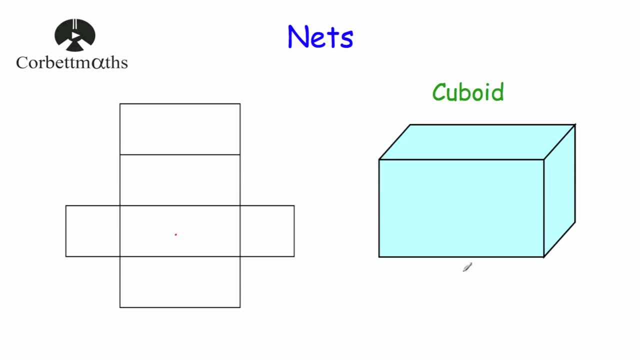 cuboid. So we've got the face at the bottom of the cuboid. this one would be the face at the bottom. this rectangle would fold up to be the face at the front of the cuboid. this rectangle would fold to be the face on the back of the cuboid. this square would fold up to be the face on the right. 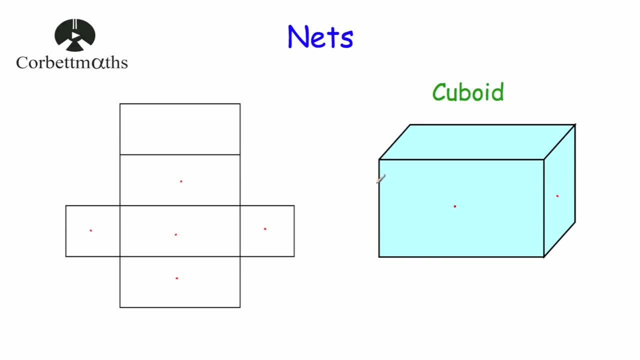 hand side of the cuboid, this square would fold up to be the face on the left hand side of the cuboid and finally, this rectangle. once you folded this rectangle up to be the back, this rectangle would fold over to be the top, the top face of the cuboid, and that's it. So that is the net of a. 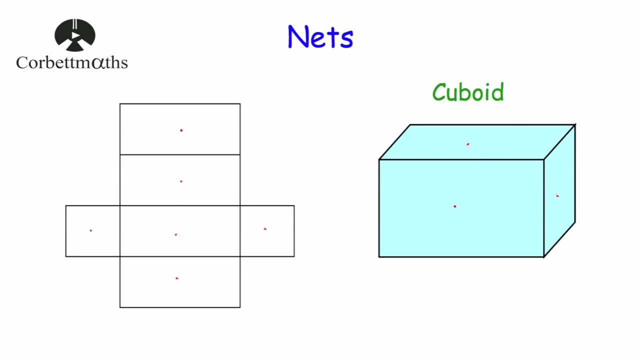 cuboid. So let's have a look at our next 3d shape and its net. So our next 3d shape is a square base pyramid. So a square base pyramid is a square base pyramid. So a square base pyramid is a square base. 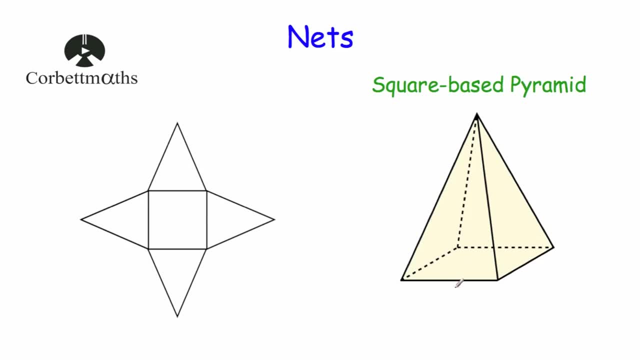 pyramid consists of a square on the bottom and then it's got four triangles that fold up to meet at the top at this apex. so here the net would look like it would have a square. that would be the base, that be the face at the bottom of. 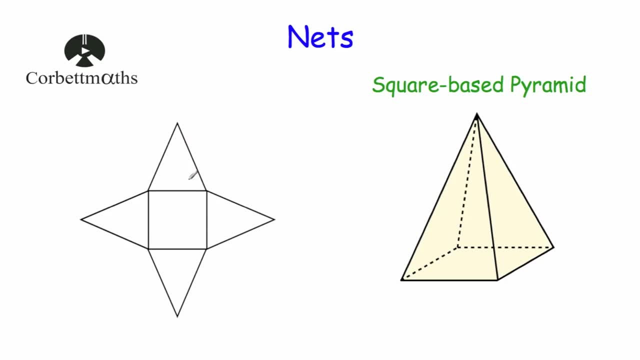 the square base pyramid, and then we would have our four triangles, and whenever you fold of those, they would all meet at the point at the top of the pyramid. so that would be the net of a square base pyramid. it would be a square with four triangles. okay, now let's have a look at a triangular prism, and it's 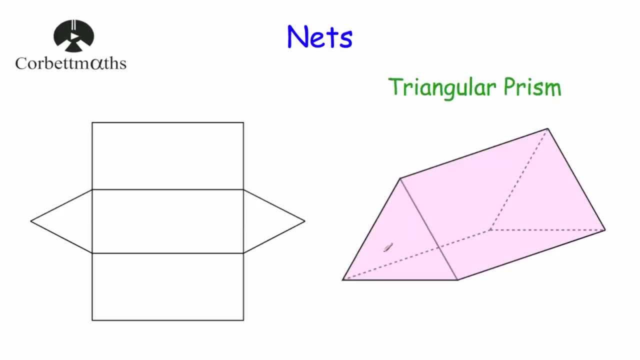 net. so here's our triangular prism. as you can see, we've got a triangle at the front of it and a triangle at the back. there we've got a rectangle on the bottom and a rectangle on the right hand side and the left hand side. so the faces. 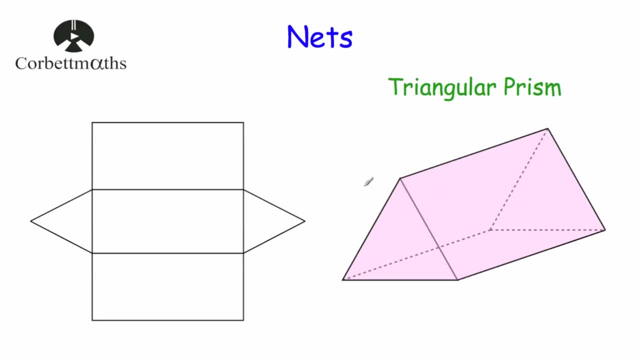 are a triangle, a triangle, a rectangle, a rectangle and a rectangle, and this would be its net, where we've got the rectangle on the base. we've then got the two triangles which would fold up to be the triangle at the front, in the back, and then we've got our two rectangles which would fold up to meet at the top off the. 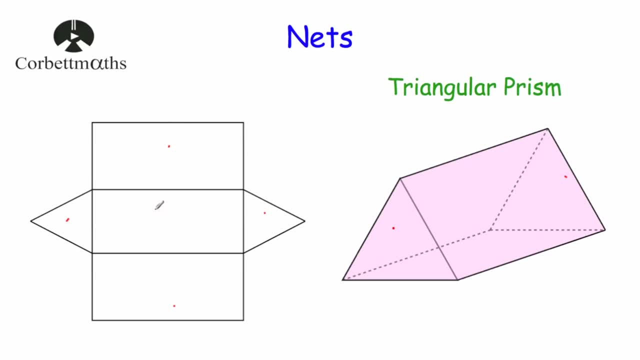 triangular prism. so this would be the net of a triangular prism, where we've got our rectangle on the base, the two triangles and then the two rectangles which would fold up to be the sides of the triangular prism. Okay, let's have a look at our next 3D ship. 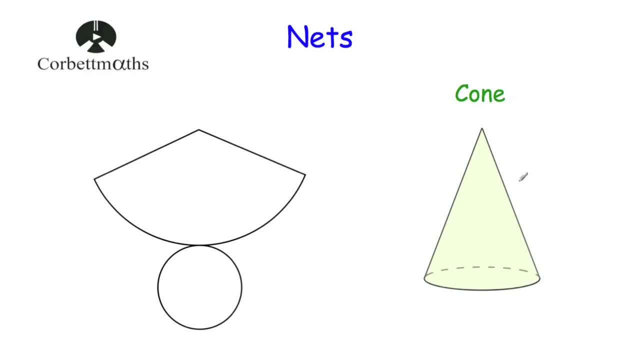 So our next 3D ship is a cone and look at its net. So this is our cone and it has got a circular base and it has got this curved face. So we have got the net of the cone, it's got the circle. 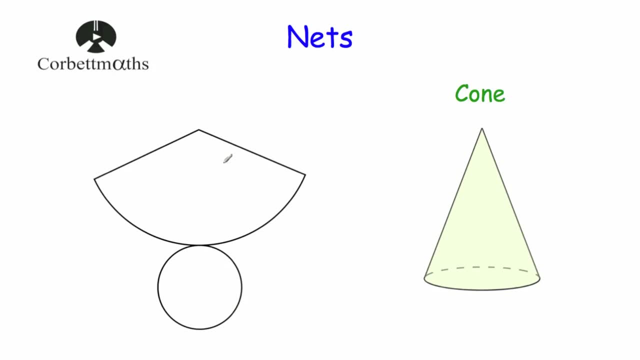 which is the circular base of the cone, so the face at the bottom of the cone, And then we've got this sector, and this sector folds around to be this curved face. So this line would join up with this line and it would fold around to be this curved face. 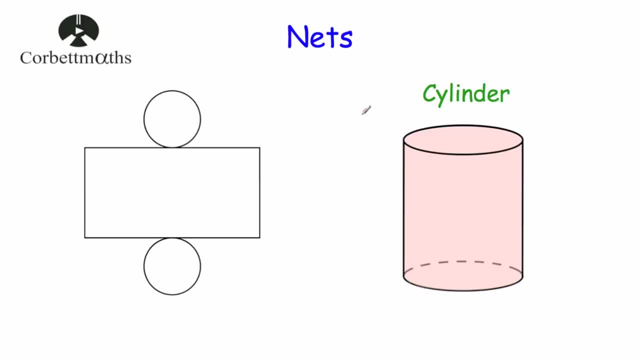 And that's it. so this is the net of a cone. So our next 3D ship is a cylinder. So here we've got a cylinder and we've got a circular face at the bottom and a circular face at the top. 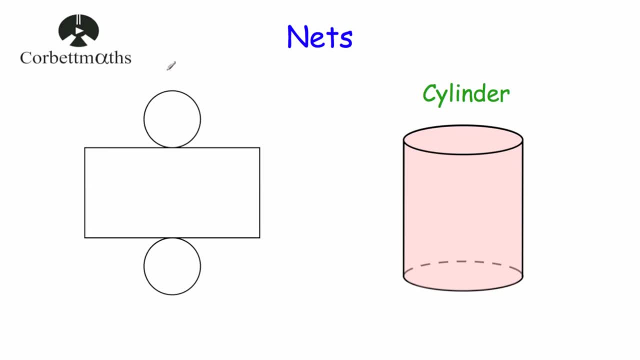 And then we've got this curved face going around the outside. And this is the net of a cylinder, where we start off with a rectangle and we roll it round and it will form the curved face going around the outside of the cylinder. 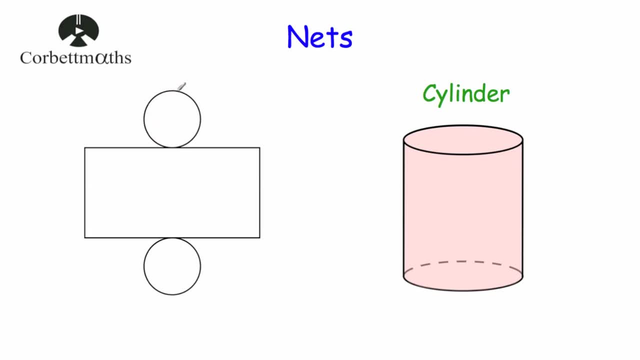 And then we've got a circle for the top and a circle for the bottom. So there are the circular faces on the top and the bottom of the cylinder. So this is the net of a cylinder, a rectangle with a circle on the top. 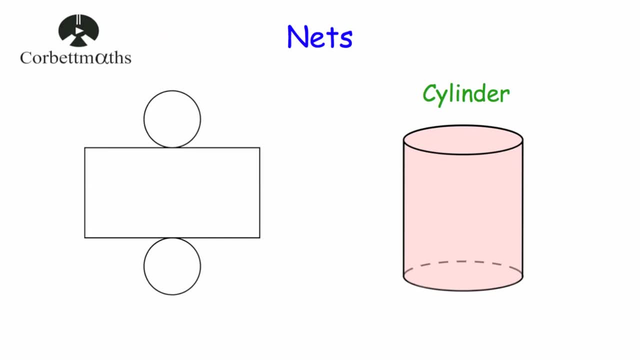 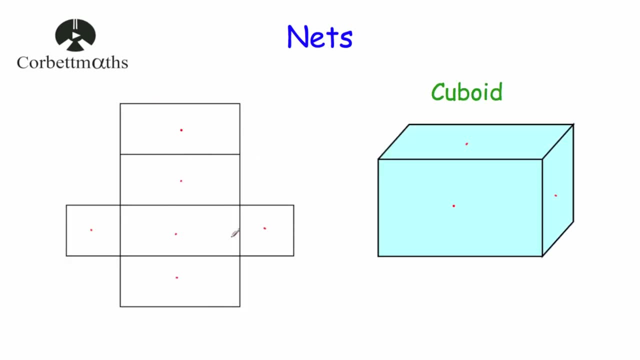 and a circle on the bottom. Okay, so we've looked at the nets of some 3D ships. so we've looked at the net of a cube, so those six squares. we've looked at the net of a cuboid, so the six rectangles, or sometimes including squares, but six rectangles. then we have got our square. 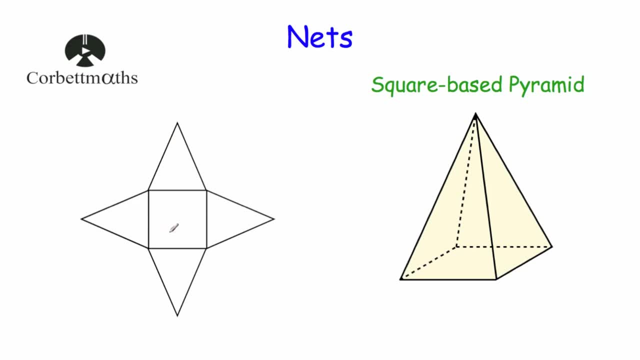 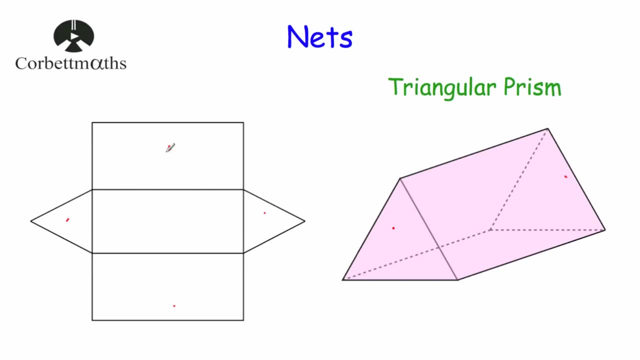 base pyramid, so that square with the four triangles is the net of the square base pyramid. we've got our net of our triangular prism, so our rectangular base, our two triangles and our two rectangles that fold up. we've got the net of a cone, so that's going to be the circle within the 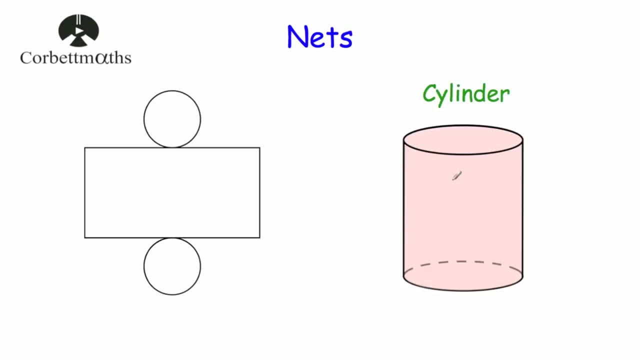 sector which folds around to be the curved surface off the cone and we've got our cylinder. so that's rectangle which folds around to be the curved face of the cylinder, with the circle on the top and a circle on the bottom. so they're the nets of some common 3d shapes. now let's have a look at some. 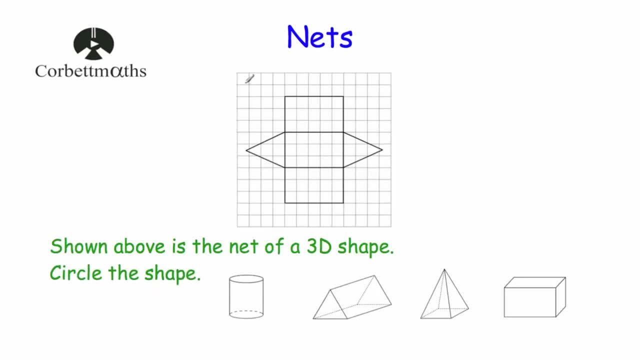 questions based on those. so here's our first question. so we've been given this grid, and on this grid is the net of a 3d shape and, as you can see, it's got two triangles and it's got a rectangle, another rectangle and another rectangle, so it's got three rectangles and two triangles. 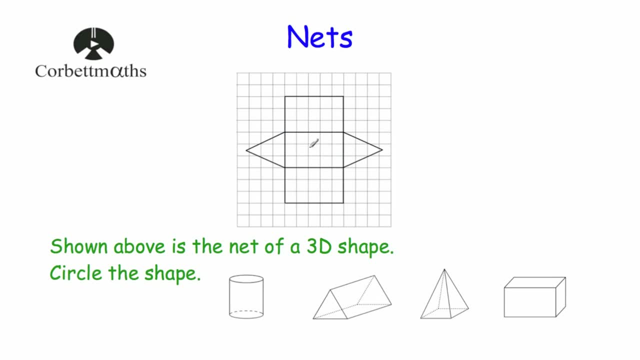 and we've been asked to circle the shape that this is the myth of seeing. see, that would be the base, with the two triangles which fold up, and then we've got the two rectangles which are full to meet at the top of the triangle, a prison that 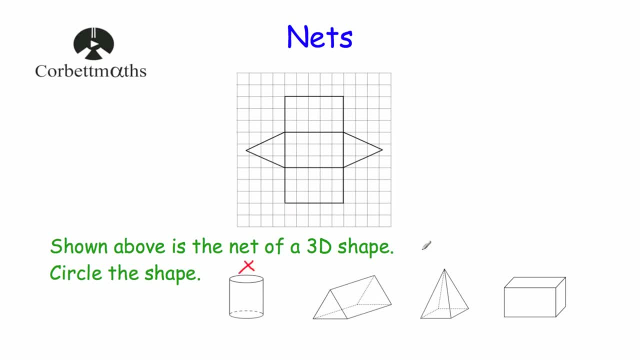 is the nerd of a triangular prism. it's not the net of a sourt�� cylinder, it's not the net of a square base pyramid, because that would be a square with four triangles, and it's not the net of a cuboid. so it's the net of a triangular prism. okay, next question. okay, let's have a look. 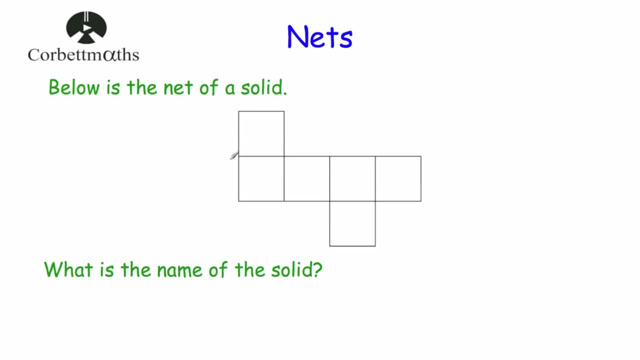 at our next question. so next question says: bluff is the net of a solid. to focus net consists of six squares. so i'm automatically thinking it's going to be the net of a cube and that will be our answer: is the net of the cube. and we're asked: what is the name of the solid? so this is the net. 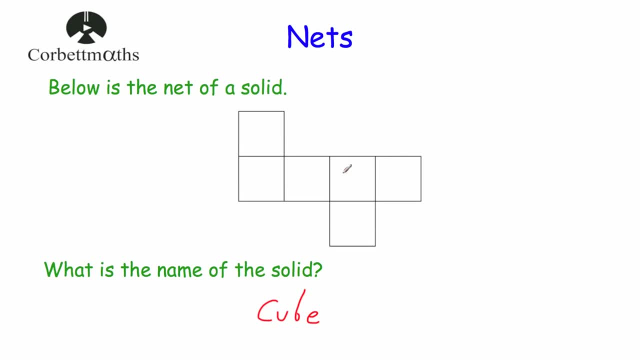 of a cube. so i'm just going to write that down. it's the net of a cube and let's have a look and see why. now this is a bit different than the net i've showed you, and there are different versions of the net of a cube, as long as they fold around to make the cube. so we have got our face on the. 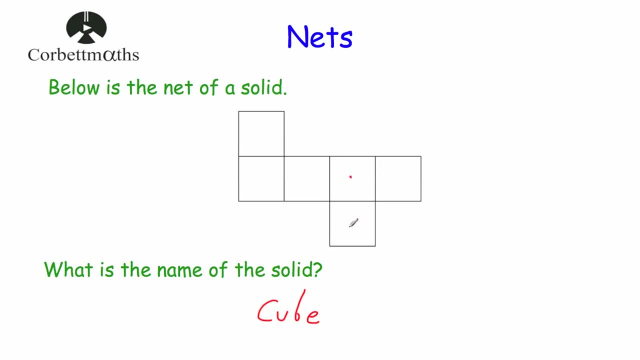 bottom of the cube. so let's call this the face on the bottom of the cube. this square would fold up to be the face of the front of the cube. this square and this square would fold up to be the faces on the sides of the cube, so the left hand face and the right hand face of the cube once this. 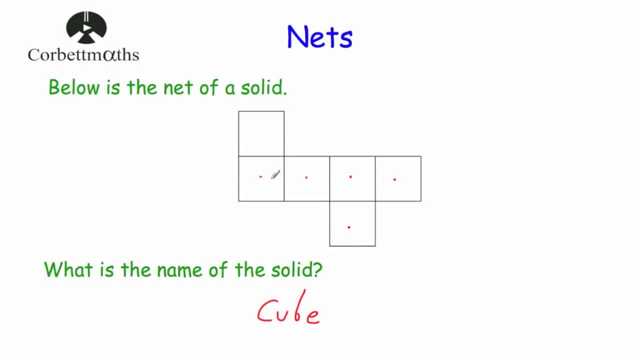 one folds up to be the left hand face of the cube, then this square would fold over to be the top of the cube, the the face on the top of the cube, and then, once this one's on top, this square would then fold around to be the face on the back of the cube. but in this question we're asked to write down the. 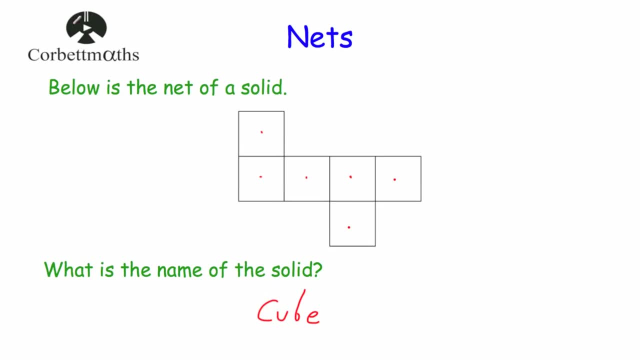 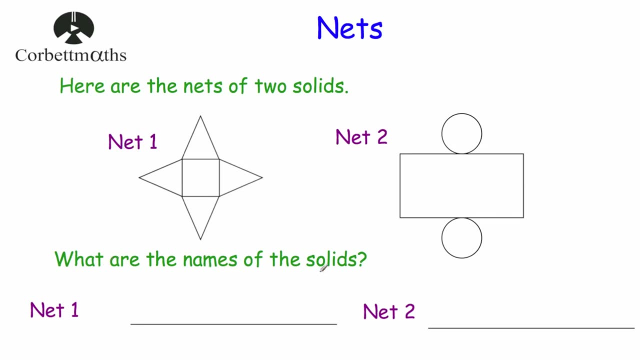 name of the solid. so the name of the solid would be a cube. so let's have a look at our next question. so next question says: here are the nets of two solids. so we've got net 1 and net 2 and we're asked: what are the names of the two? 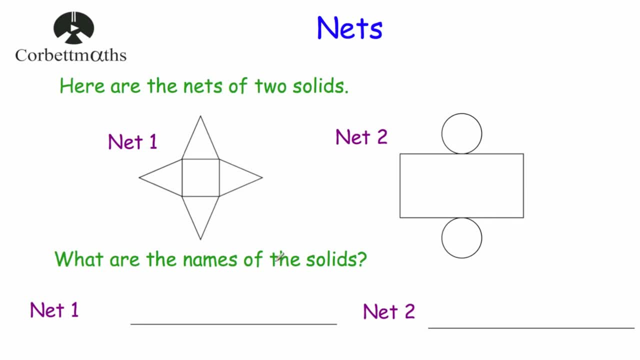 solids. so, in other words, whenever we fold up these nets, what 3d shapes will we make? so this net, net 1, that is the net of a square base pyramid, we've got our square base and then we've got our four triangles which fold upwards. that 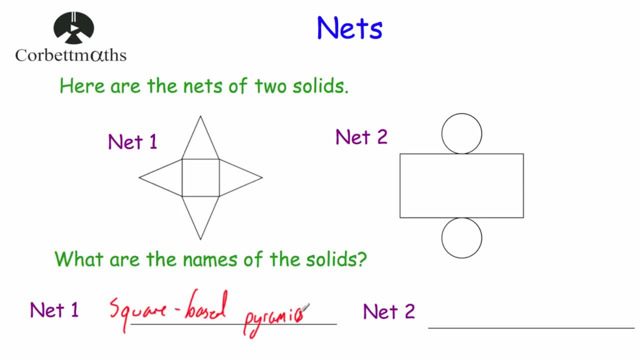 is a square base pyramid and our next net. well, this net is the net of a cylinder. we've got our rectangle, which folds round to be that curved face off the cylinder, and then we've got the circle for the top and the circle for the base, so that is going to be the net of a cylinder. okay, okay, let's have a. 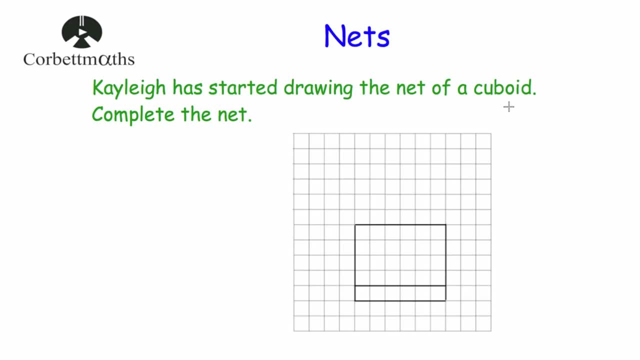 look at our last question. so last question says Kaylee has sort of drawn the net of a cuboid, complete the net. so this is the start of the net of a cuboid and we've been asked to complete the net of the cuboid. we know it's not. 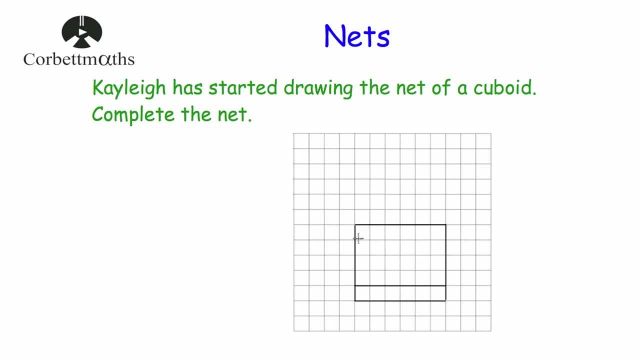 complete because there's only two rectangles. we're going to need six. so we have got this rectangle, this larger rectangle. I'm gonna let that be the base of the cuboid. so that's gonna be the base of my cuboid and it is a rectangle and it's one, two, three, four, five, six squares along. 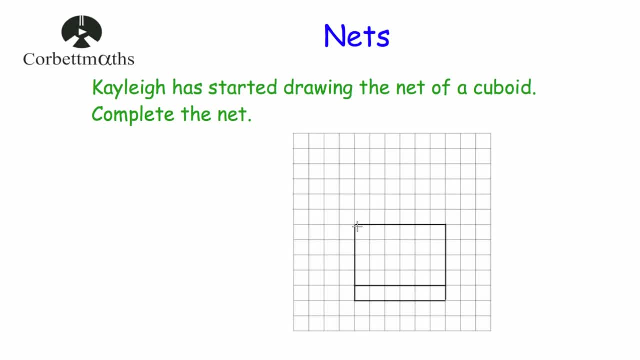 and it's one, two, three, four squares wide. so it's a six by four rectangle. and then we've got this rectangle. I'm gonna say that's the front face of the cuboid. so whenever I fold this rectangle upwards, it's going to be the front face. 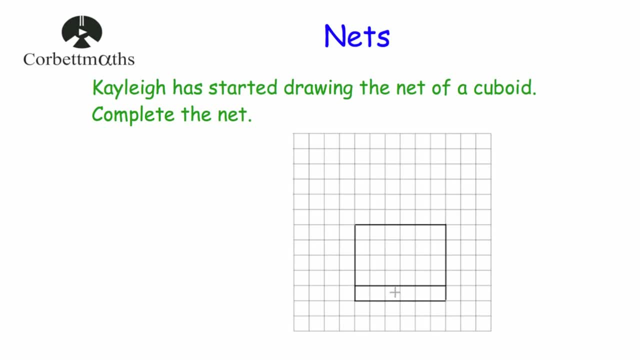 and it is a six by one rectangle. so that's gonna be the front face. this is the base. I'm not gonna draw the back face off the cuboid, so the the face on the back of the cuboid. so that's gonna be the same as the front. so it's gonna 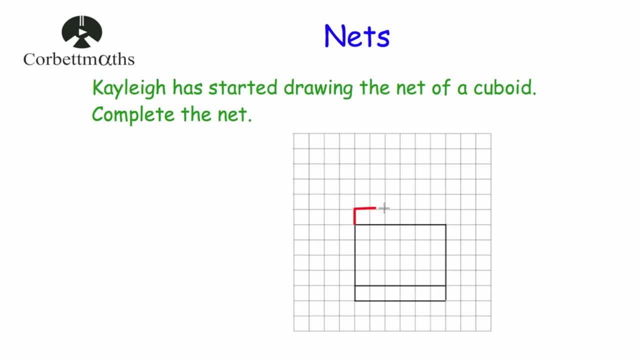 be a six by one rectangle as well. so six by one, so one up and six across, and then we would have our base and we would have the face on the back of the cuboid and the face on the front of the cuboid. now we've got our base, our back and our front. now let's get the top, the lid. 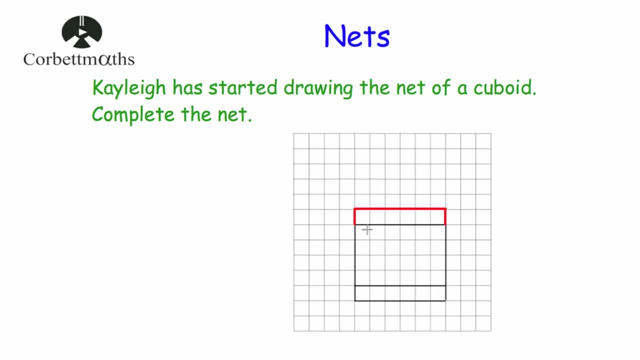 of the cuboid. so i'm going that'll be identical to the base of the cuboid. so it's going to be a six by four rectangle as well. so let's draw that above here. so one, two, three, four and six across, like so, and that would be the base, the front, the back and the lid of the cuboid. so we've now got. 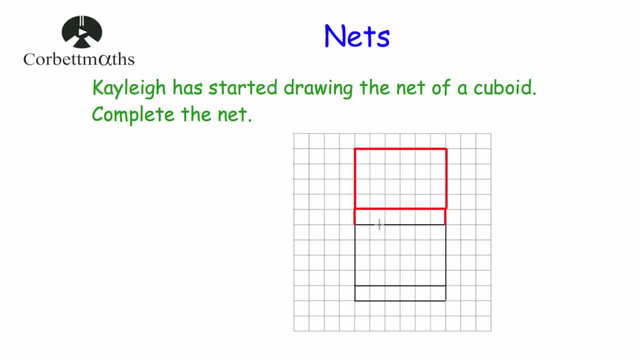 four of the faces. we just need two more faces: the left hand face and the right hand face. so if we go back to our base, we're going to need a face that is on the left hand side and the right hand side and whenever we fold up the front and the back, you can see the cuboid would have a height.